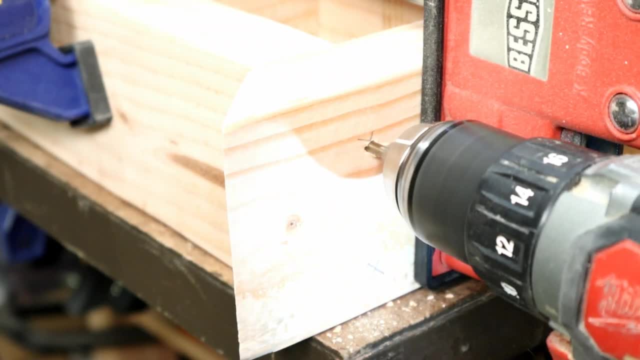 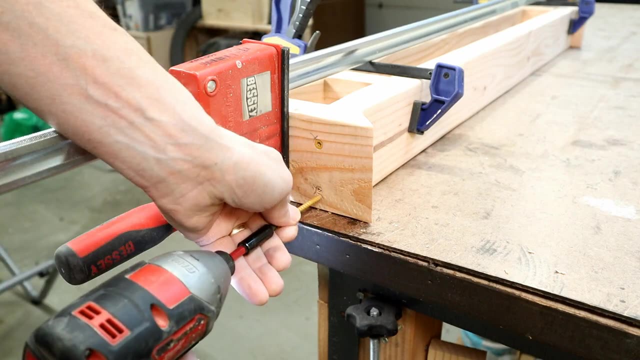 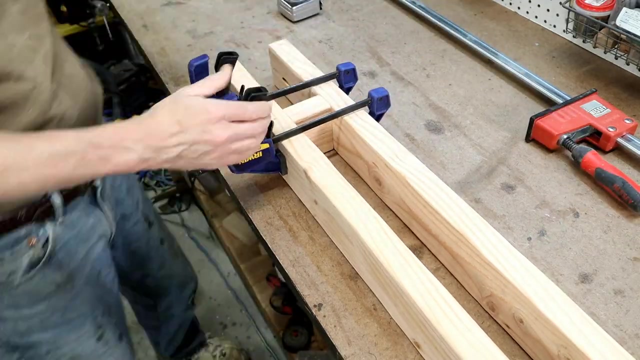 the top end to clamp it in place. I pre-drill for four two and a half inch deck screws, two on each side going into the leg. I place the top spacer down seven and a half inches from the top. I clamp and put one screw on one end of each side. it's really secure and it's one less screw. 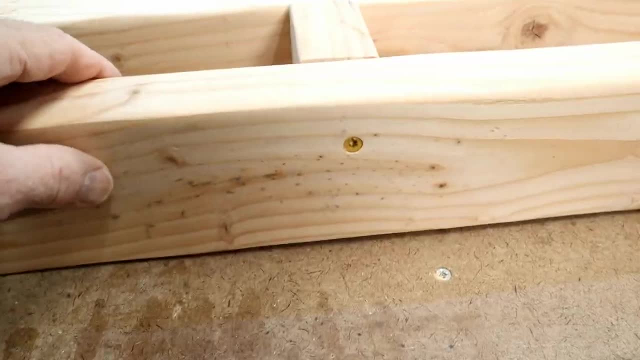 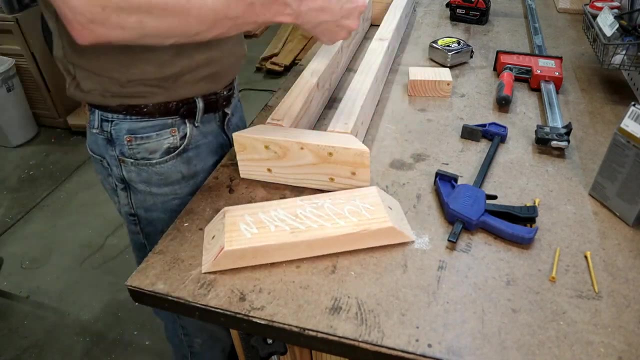 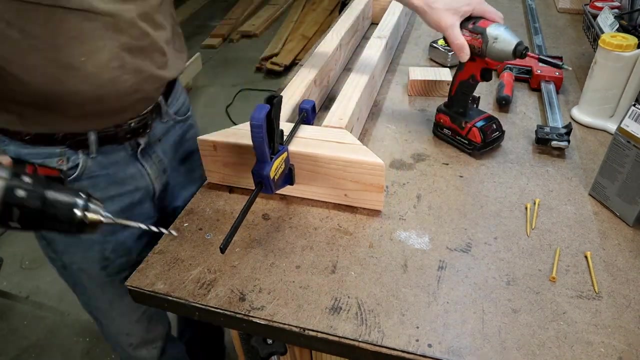 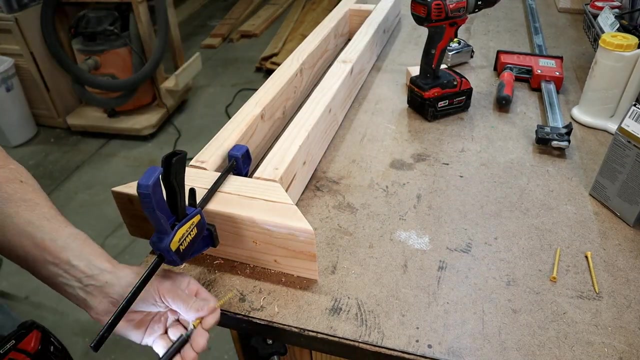 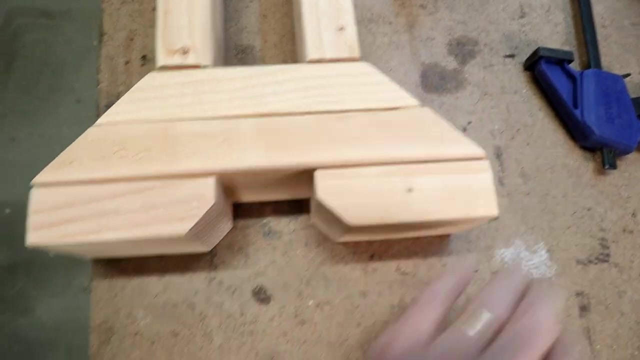 hole to fill with putty. now I glue, clamp and screw in the bottom piece of the leg assembly. this piece also has 45 degree angle cuts on both ends and it is eleven and a half inches long point-to-point. next up are the feet. they are four and a half inches long with the bottom inside corner cut at a. 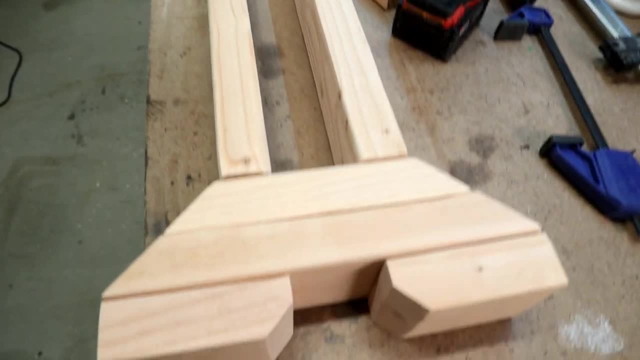 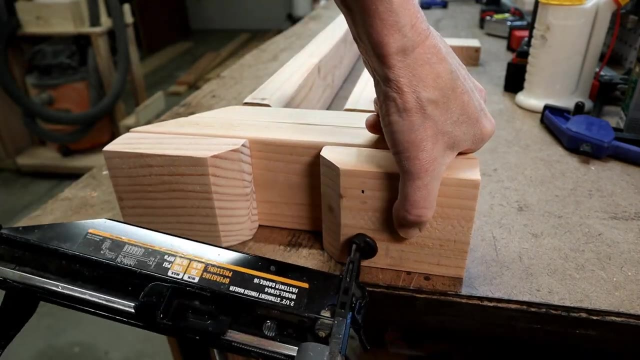 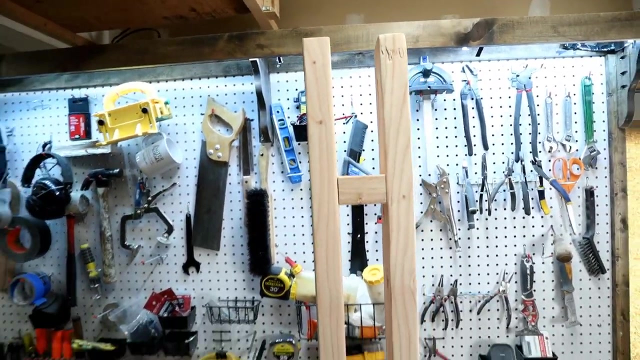 45 degree angle and positioned as shown. I glue a nail at each corner, making sure I'm far enough in on the outside edge so the nail doesn't come out the other side. now the first leg assembly is finished, I'll show the second one, uninterrupted so. 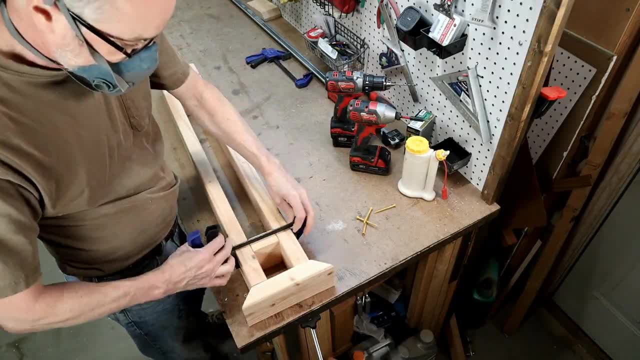 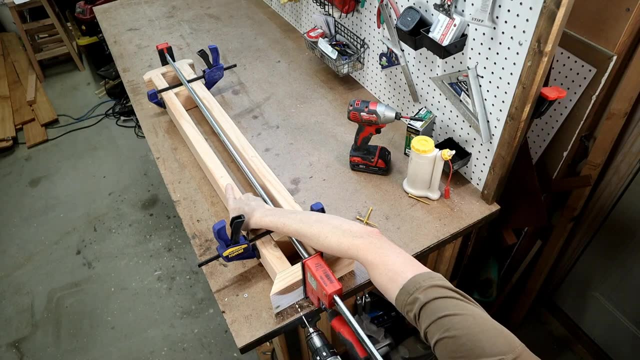 you'll get a better idea how simply and quickly this can go now. in this one I wound up doing the feet before the top stretcher block, but it really doesn't make a difference. I'll show you how to do the feet before the top stretcher block. 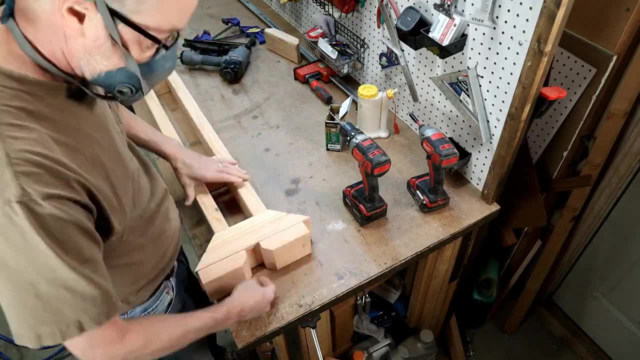 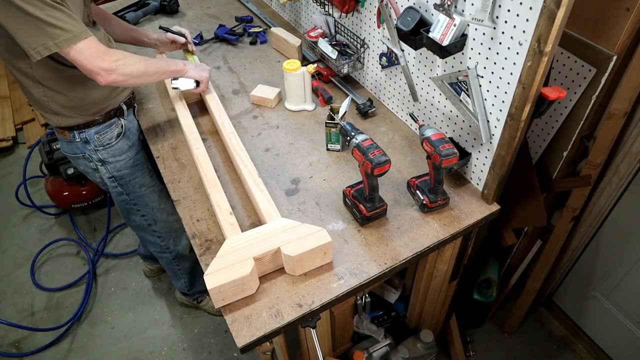 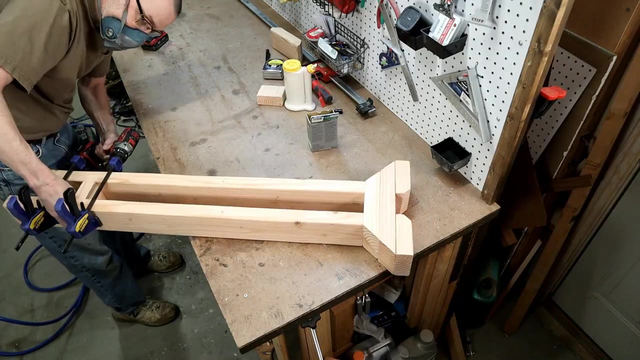 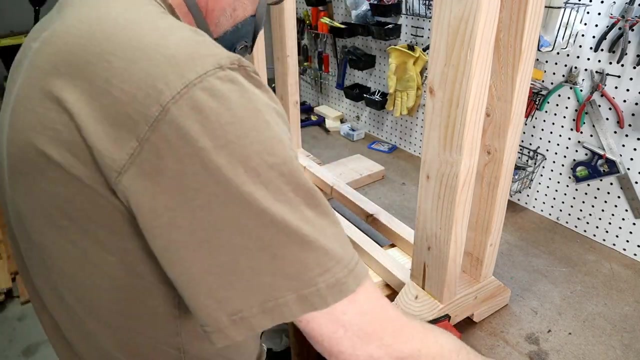 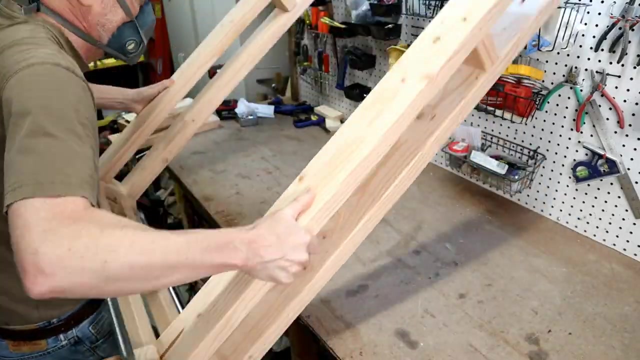 the next thing I do is install the bottom stretchers with the pocket holes facing down. I line them up with the legs so they should be five and a half inches from outside edge to outside edge. there are several ways you can do this, of course, depending on your workstation. 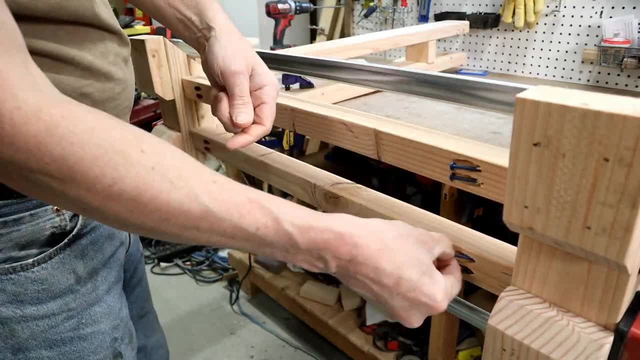 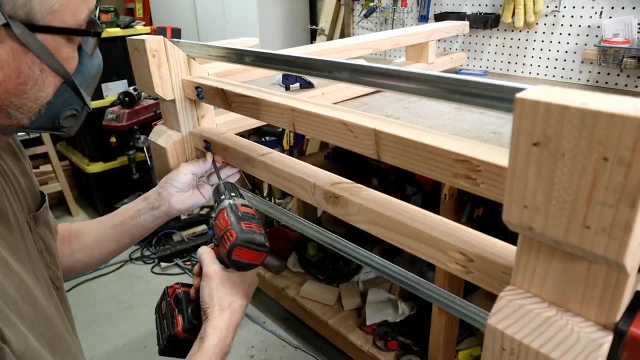 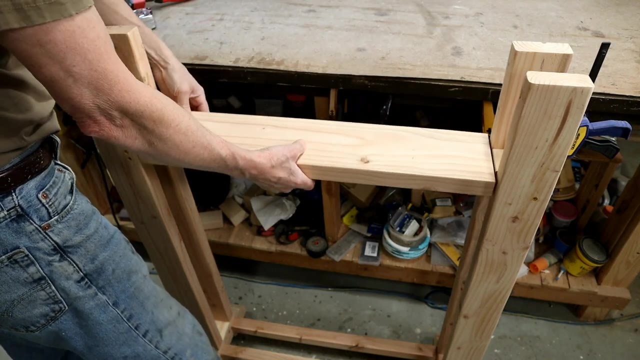 I just think on the fly and clamp this to my bench. it gets the job done here. I've clamped some wood under the spacer so I can lay the shelf in and have it line up with the spacer blocks. then I clamp and screw in the pocket hole screws. 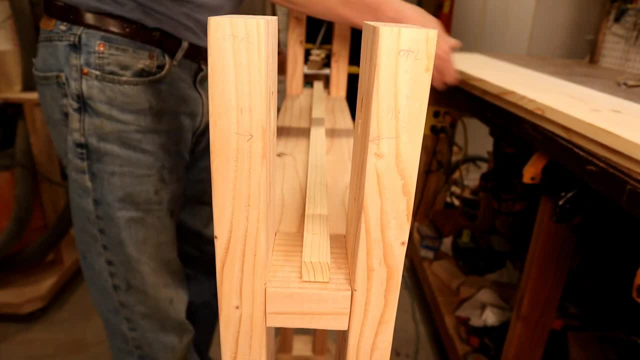 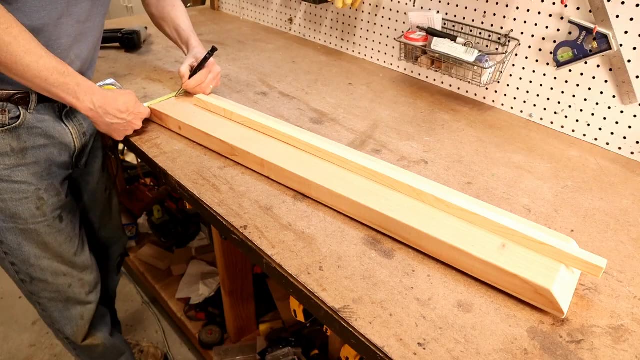 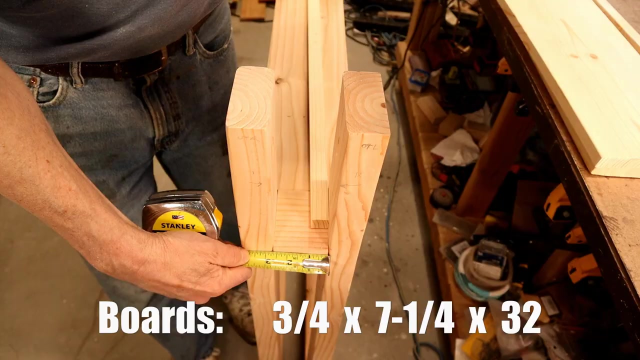 now here's the hidden feature I talked about earlier. I place a three-quarter inch square rail in the middle of the shelf as well as in the middle of the bottom side of the top board, and that leaves me room for two sign boards to slide in, giving a total of four possible signs to have on hand. 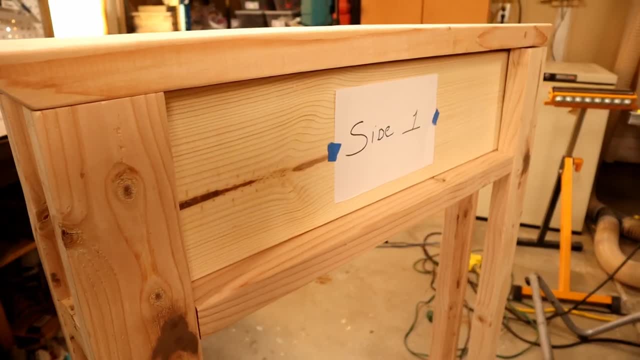 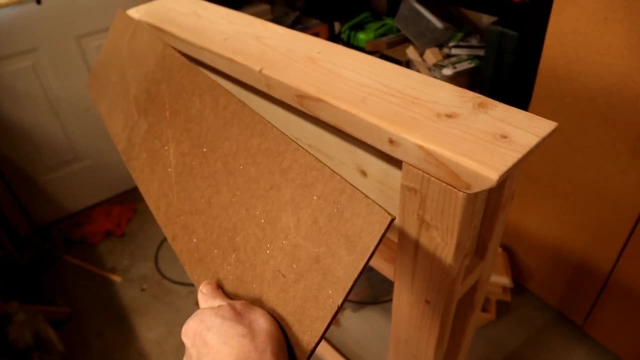 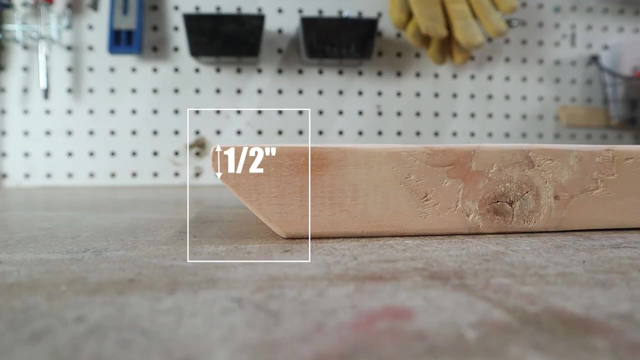 now, if you don't want the lantern lights, you could use this as a reversible stand and flip it around to show side two. you could even replace the two three-quarter inch thick boards with six quarter inch ones and have twelve sides. the top is a two by six. that is 35 inches long, and I cut a 45 degree angle on the underside. 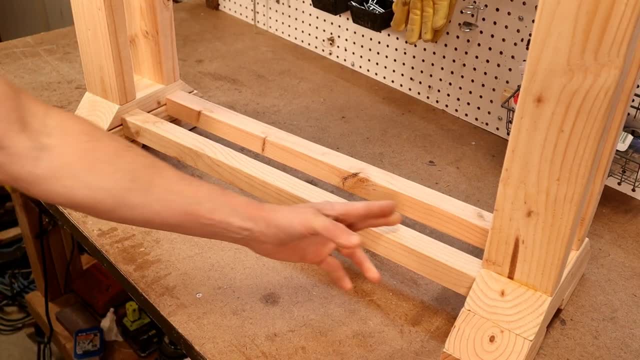 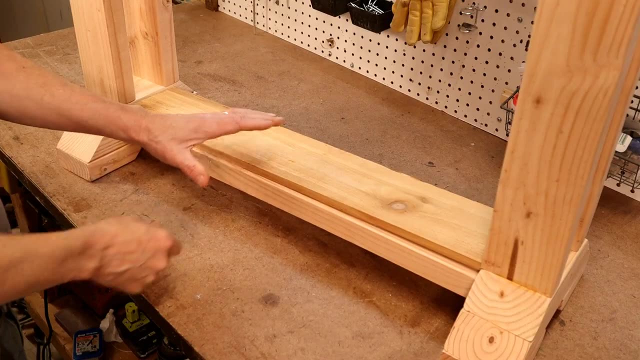 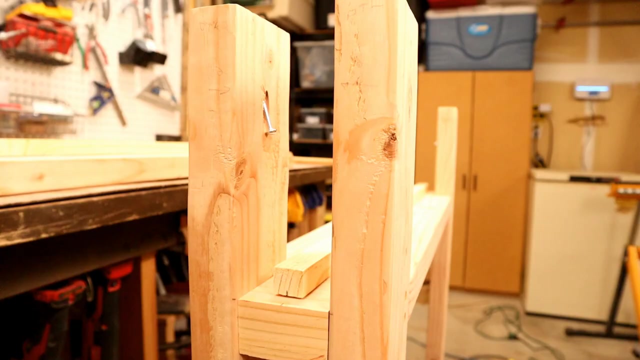 of each end, as shown here. as far as the bottom stretchers go, you can leave them as is. you could put a board on top, or you could put slats on, like I'm going to do with this one. use your imagination and come up with your own twist. now, when, 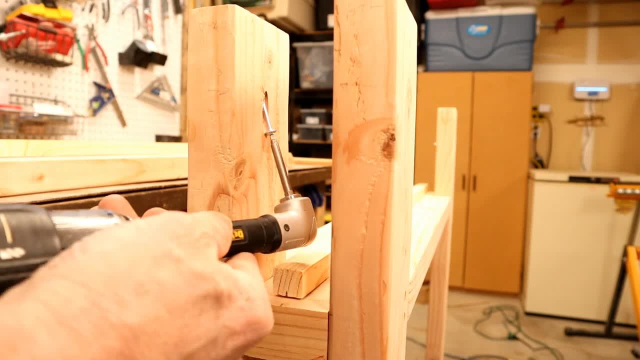 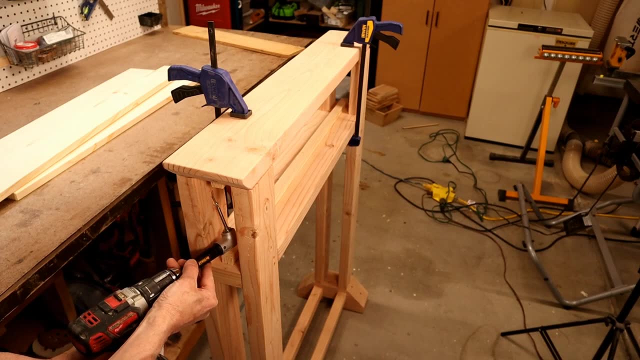 you're ready to screw in the top there won't be much room, but you can still access the screws with a right angle adapter for your drill. I use this DeWalt one all the time and I love it. here I'm going to show you how I painted. 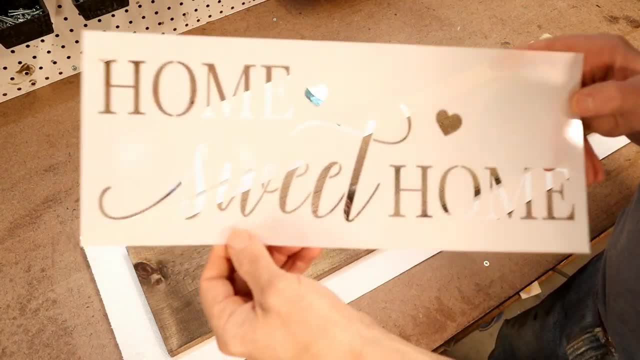 the two signs I've done so far. I use stencils like this one- cinderella- and the other one are the same. I'm going to show you how I painted the two signs I've done so far. I use stencils like this one: cinder. 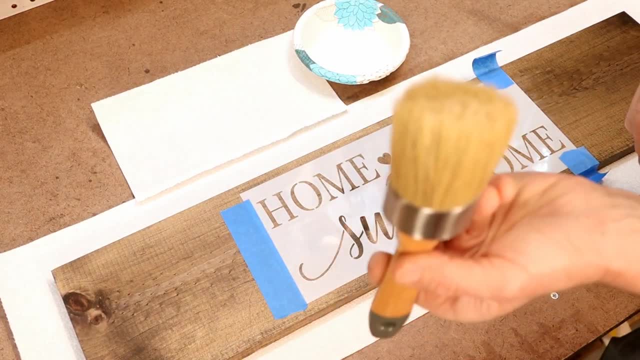 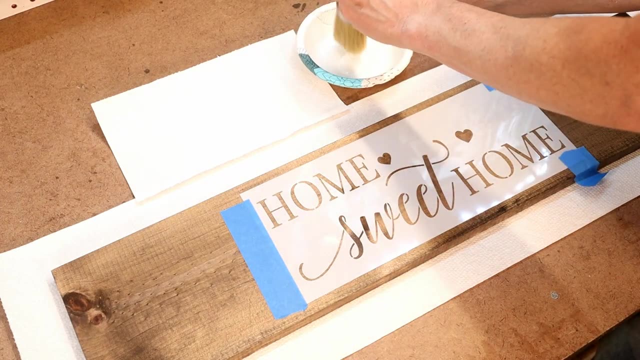 it on the board and use painters tape on each end to secure it. then I use a round brush. this one is milk paint brush. I lightly dip it in the paint, wipe the brush on a paper towel to get most of the paint off and lightly dab the paint. 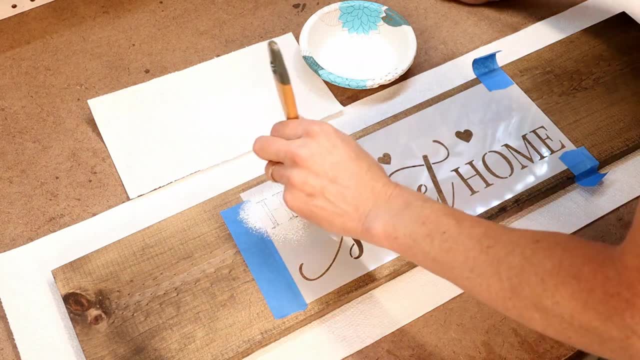 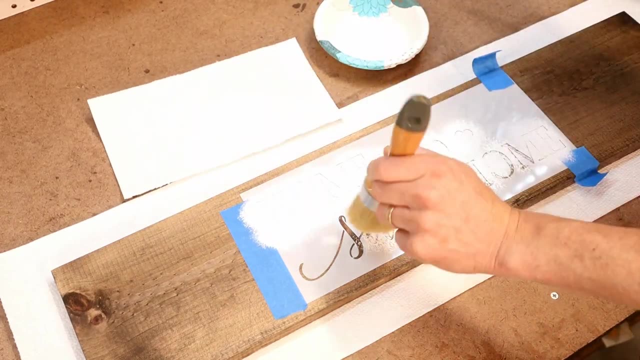 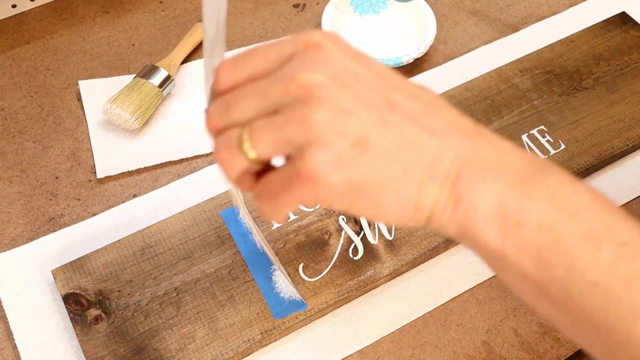 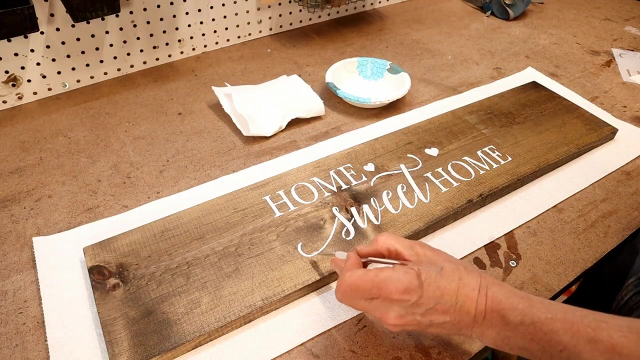 onto the stencil straight up and down. this helps prevent bleed through. make sure you have good coverage. be careful not to dab on the outside of the stencil and when you're finished, slowly peel the stencil up and away. if you want, you can get a thin brush and outline the letters. I had a 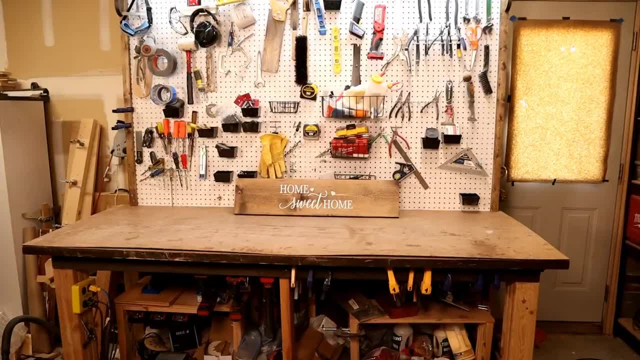 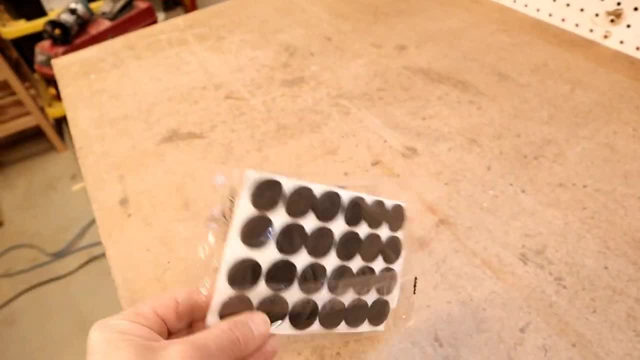 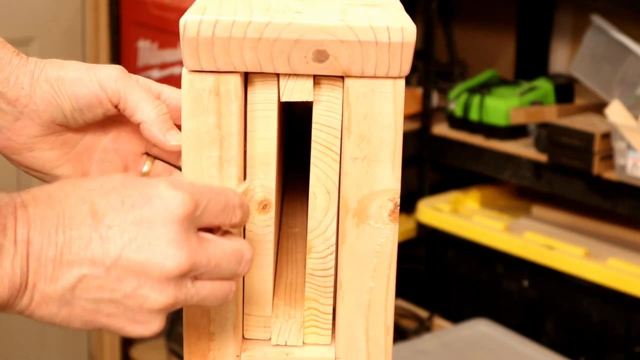 little bleed through, but you can't really tell from a distance and I can live with it. I put these rubber pads on the bottom of the feet to protect from ground contact. if the boards are a little loose you can put a shim in to tighten them up so they don't rattle in the wind.